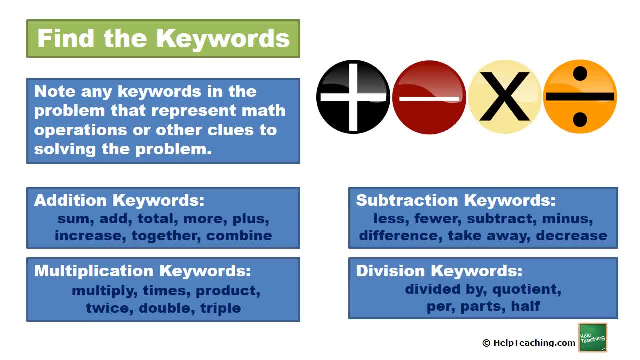 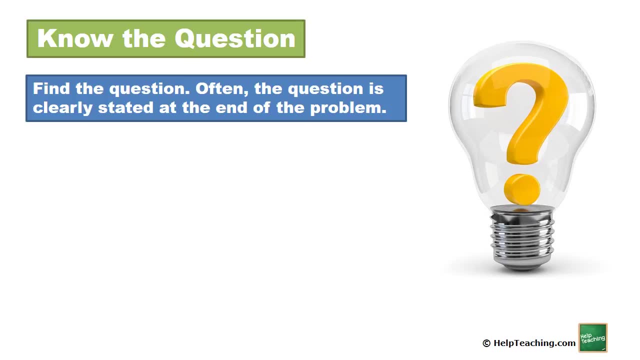 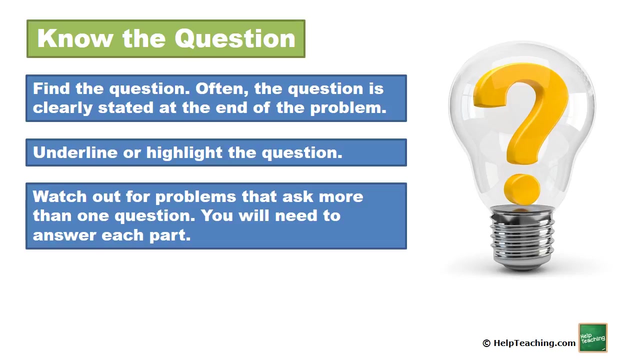 Division. key words include: divided by quotient, per parts and half. Know the question. Find the question. Often, the question is clearly stated at the end of the problem. Underline or highlight the question. Watch out for problems that ask more than one question. 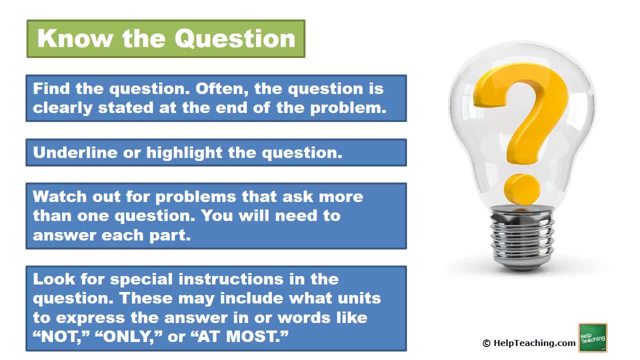 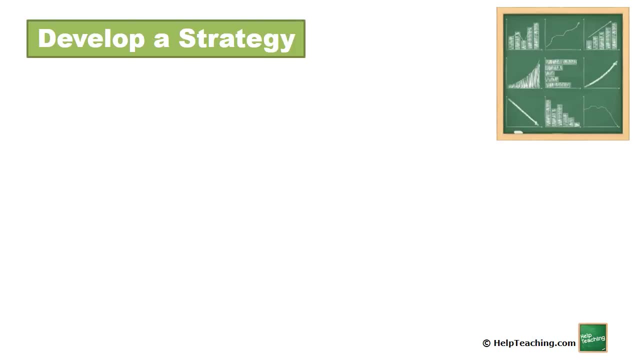 You will need to answer each part. Look for special instructions in the question. These may include what units to express the answers in, or words like, not only, or at most, Develop a strategy. If there is a figure, table, graph or other visual information in the problem, use it. 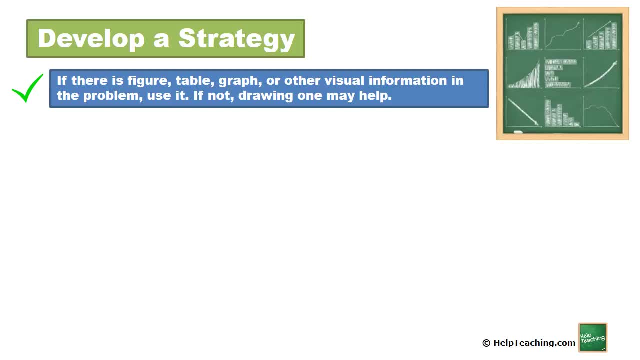 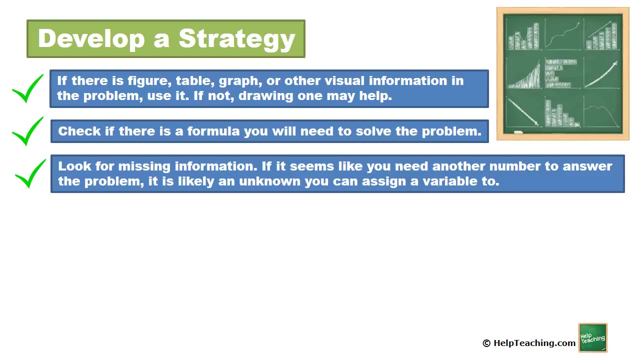 If not, drawing one may help Check. if there is a formula you will need to solve the problem. Look for missing information. If it seems like you need another number to answer the problem, it is likely an unknown. you can assign a variable to. 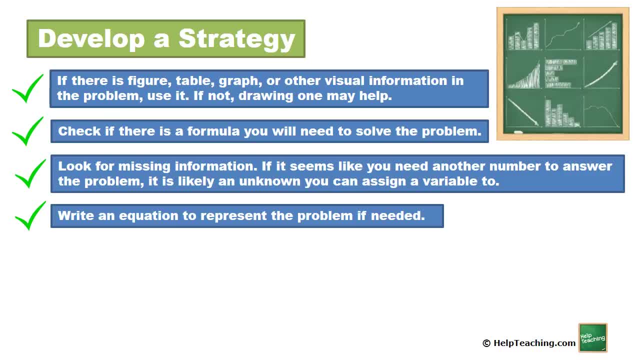 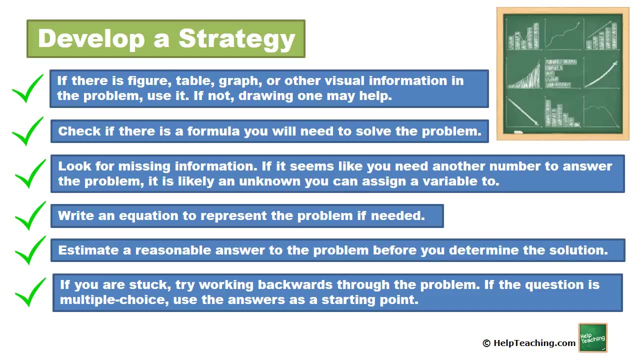 Write an equation to represent the problem. if needed, Estimate a reasonable answer to the problem before you determine the solution. If you are stuck, try working backwards through the problem. If the question is multiple choice, use the answers as a starting point. Solve the problem. 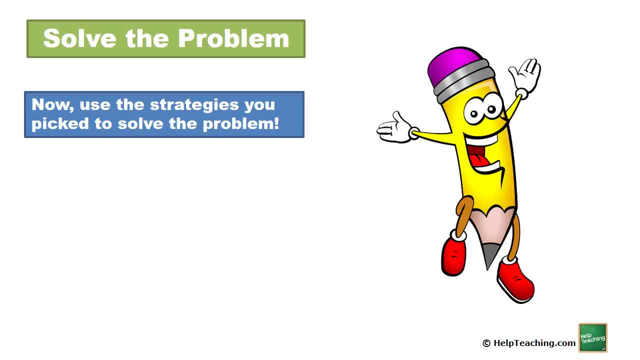 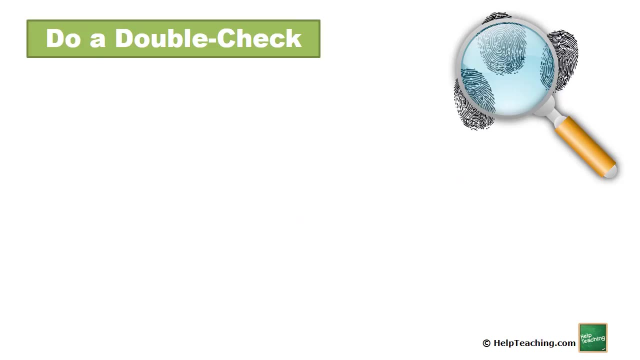 Now use the strategies you picked to solve the problem. Write out each step of your work, Show your calculations. Be sure to label your answer with units if necessary. Do a double check. Re-read the question. Did you answer the right question? 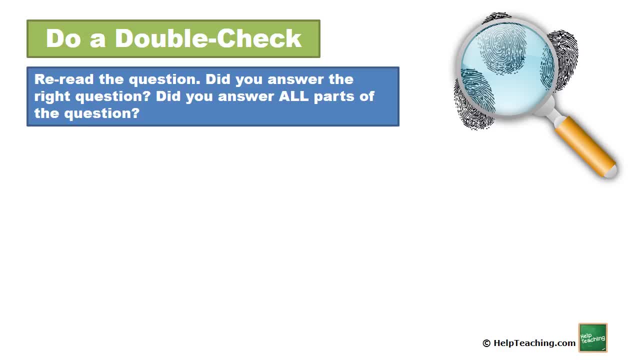 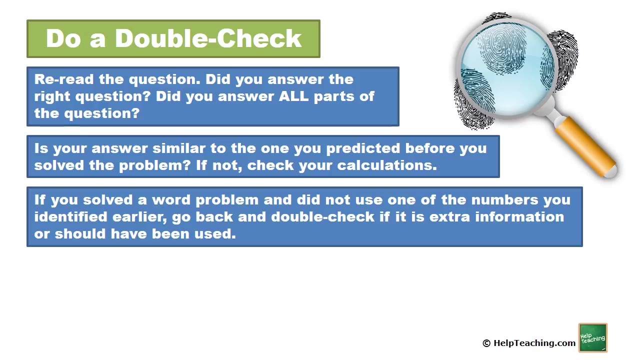 Did you answer all parts of the question? Is your answer similar to the one you predicted before you solved the problem? If not, check your calculations. If you solved a word problem and did not use one of the numbers you identified earlier, go back and double check if it is extra information or should have been used. 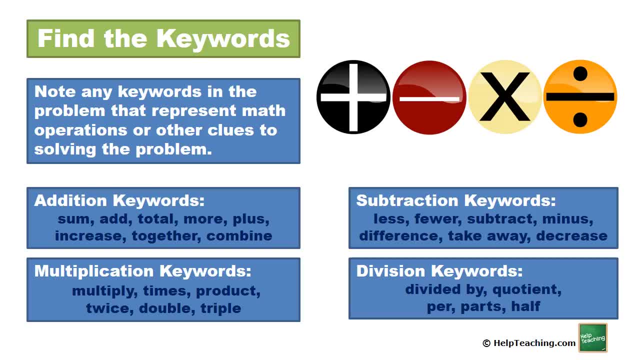 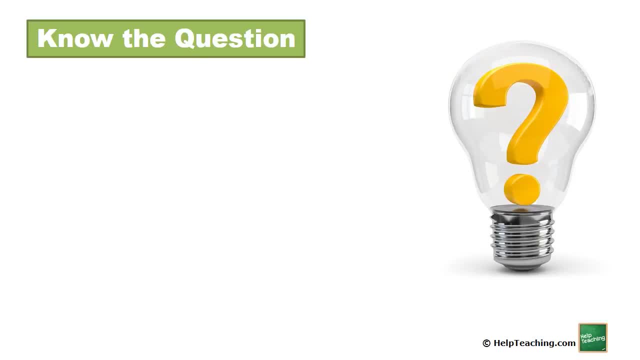 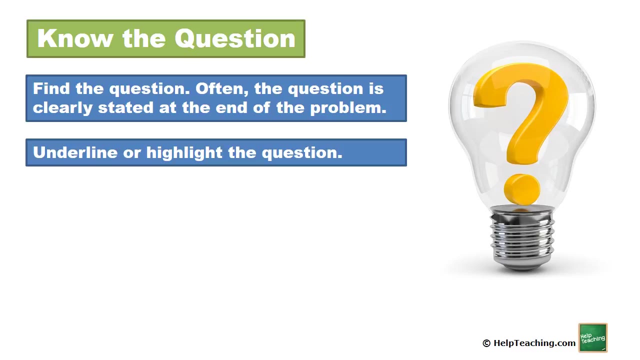 Division. key words include: divided by quotient, per parts and half. Know the question. Find the question. Often, the question is clearly stated at the end of the problem. Underline or highlight the question. Watch out for problems that ask more than one question. 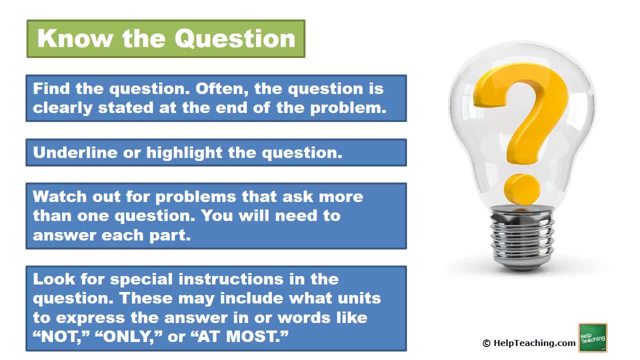 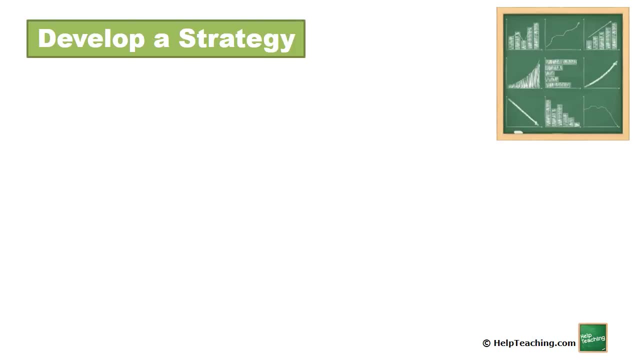 You will need to answer each part. Look for special instructions in the question. These may include what units to express the answers in, or words like, not only, or at most, Develop a strategy. If there is a figure, table, graph or other visual information in the problem, use it. 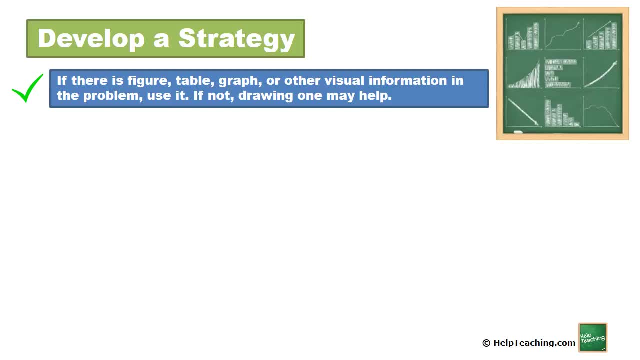 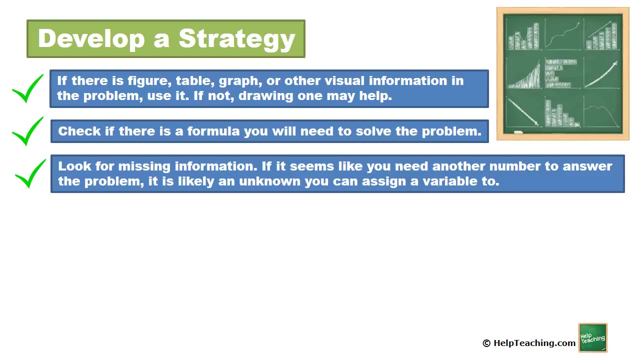 If not, drawing one may help Check. if there is a formula you will need to solve the problem. Look for missing information. If it seems like you need another number to answer the problem, it is likely an unknown. you can assign a variable to. 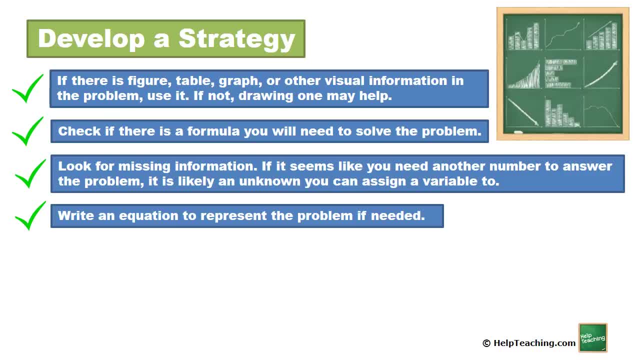 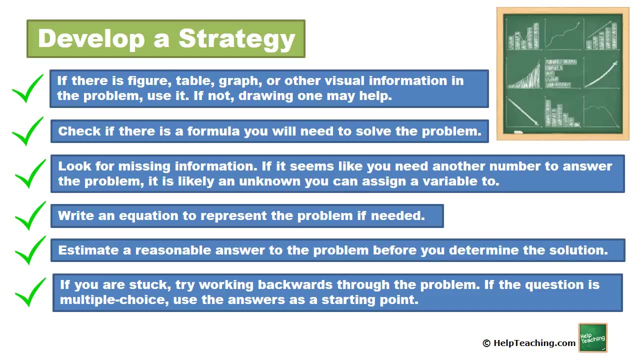 Write an equation to represent the problem. if needed, Estimate a reasonable answer to the problem before you determine the solution. If you are stuck, try working backwards through the problem. If the question is multiple choice, use the answers as a starting point. Solve the problem. 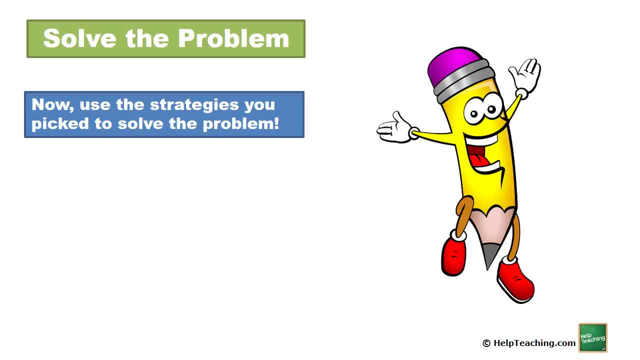 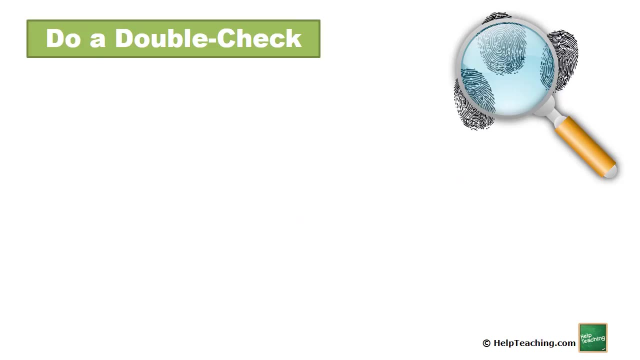 Now use the strategies you picked to solve the problem. Write out each step of your work, Show your calculations. Be sure to label your answer with units if necessary. Do a double check. Re-read the question. Did you answer the right question? 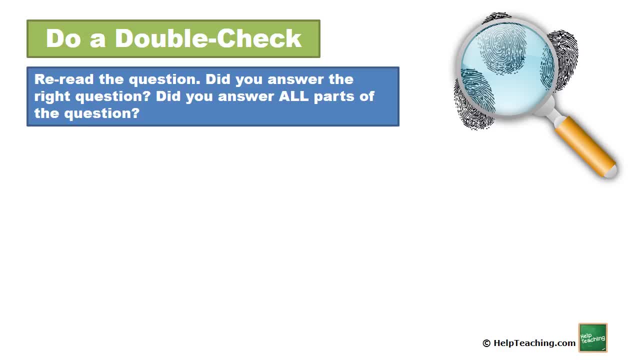 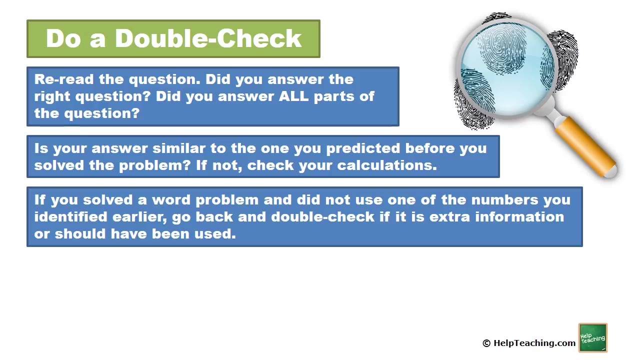 Did you answer all parts of the question? Is your answer similar to the one you predicted before you solved the problem? If not, check your calculations. If you solved a word problem and did not use one of the numbers you identified earlier, go back and double check if it is extra information or should have been used.